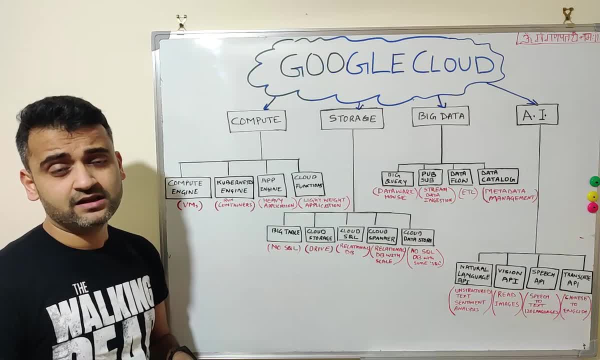 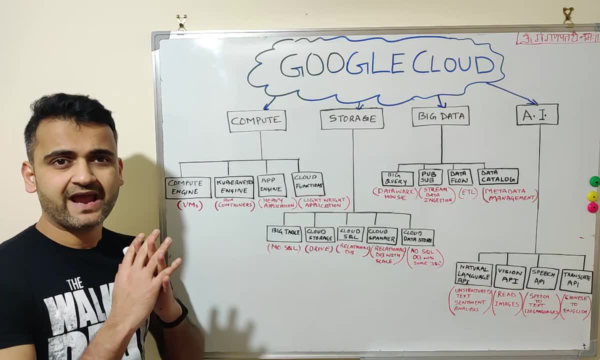 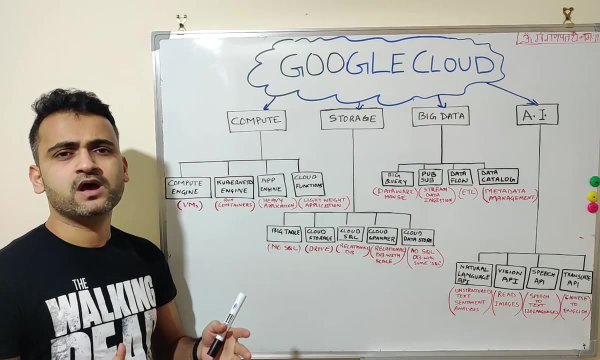 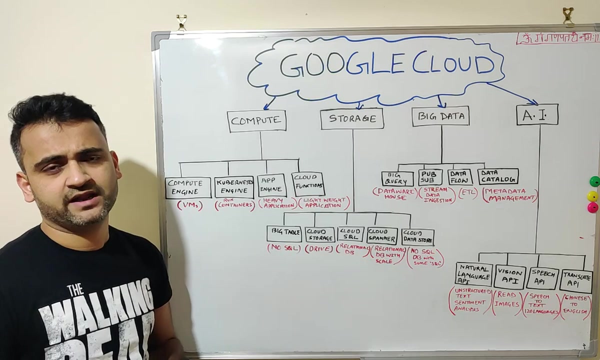 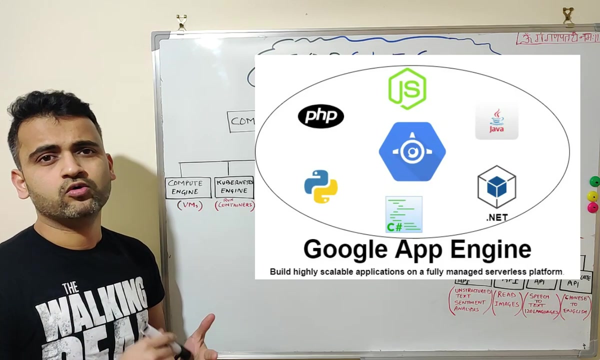 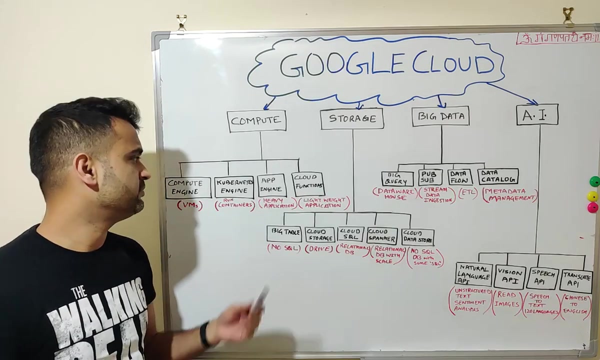 moving on app engine, as the name suggests, again, it is an application engine where you can deploy your web applications, your large scale applications, without any headache of managing the back-end infrastructure. so suppose you want to develop a customized website for your customer which runs a business- choose product, supplier and you need not have any. 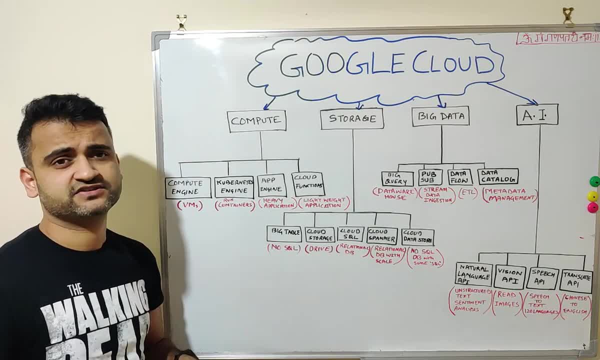 cloud to seguely resolve this. our best way to execute productın in-house y on go, python, javanet- all these languages can be used and that application can be developed and that can be easily deployed and scaled on app engine. you have to spend nothing on infrastructure. it is a managed service where all the infrastructure is managed by google cloud from the backend. cloud functions, also on similar lines, works pretty much similar to an app engine. so cloud functions and app engines are quite similar. but what is the basic difference? cloud function also lets you deploy your application on to it, but it is meant mostly for single-purpose, lightweight application, whereas an app engine is meant for complex and large-scale applications. so 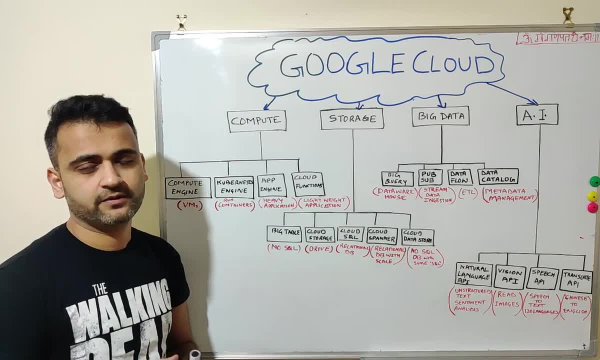 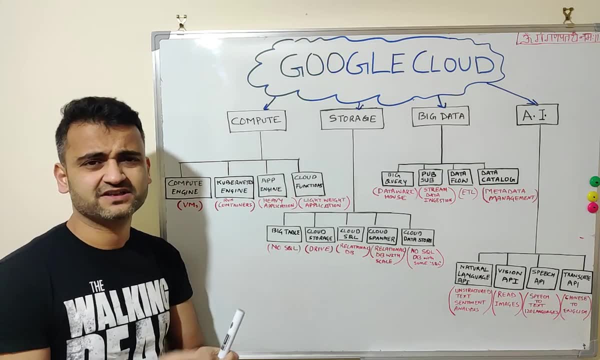 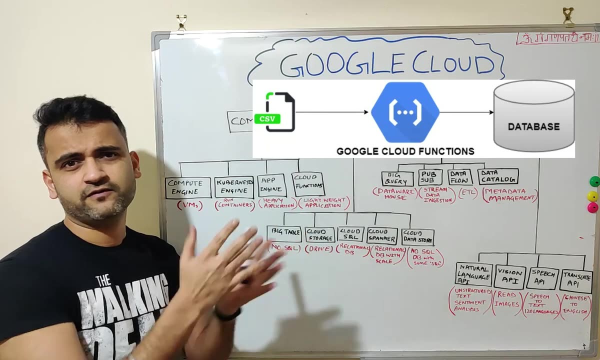 suppose, if your application has various modules integrating with each other, then an app engine is a correct product for you. but if you want to deploy a single purpose function- suppose if you have, if you want to write a program which fetches the data from from one of your drives and from your CSVs, runs it. 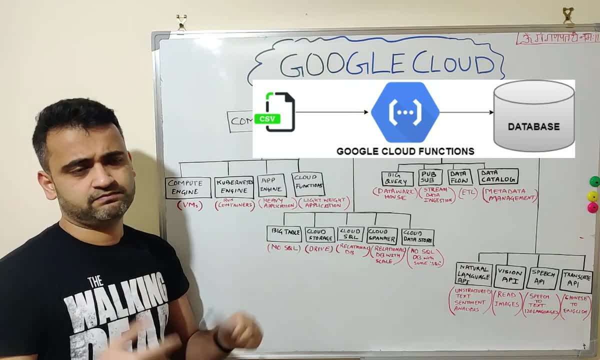 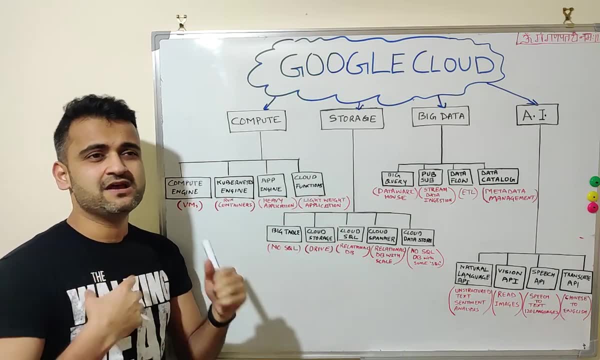 messages, that data and then load it into a database, then mainly, you are focusing on something like cloud function, because it is a lightweight technology which can quickly help you deploy your single purpose function. so that is, you are focusing on something like cloud function because it it is a lightweight technology which can quickly help you deploy your single-purpose function. so that is. 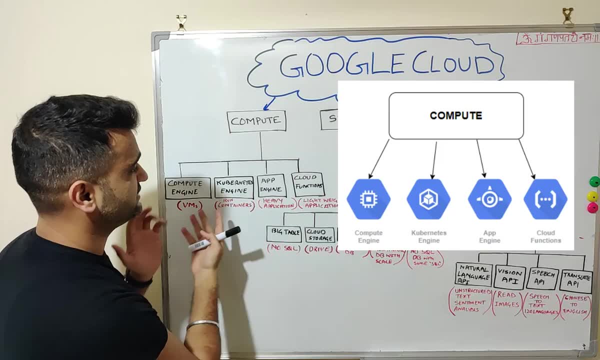 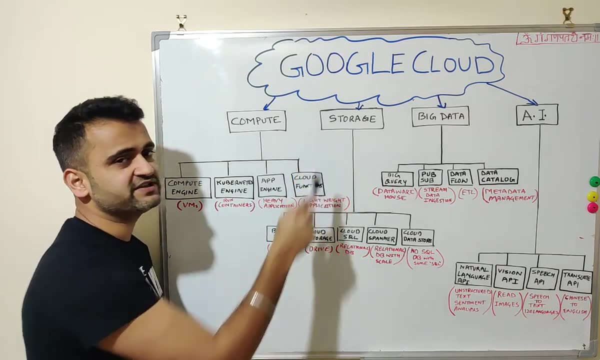 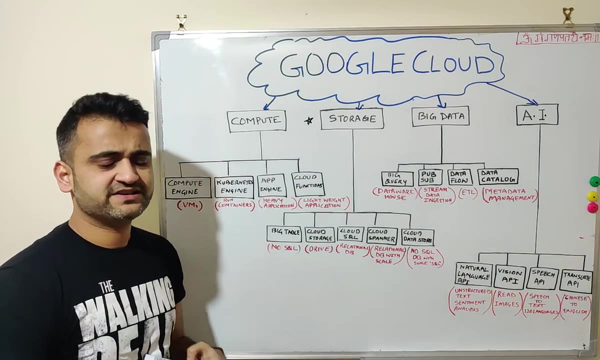 is your whole overall compute platform, and these are the four major services provided under this category. moving on storage, now this is the usp of google cloud because ever since google came into the market, its storage- how it processes the data- has always been its usp under google. 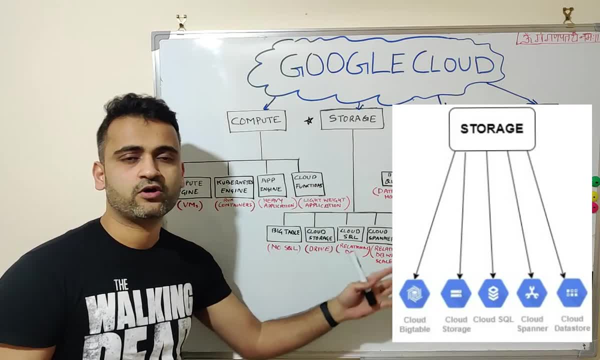 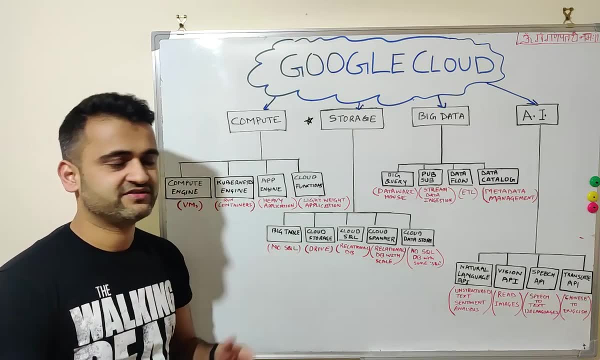 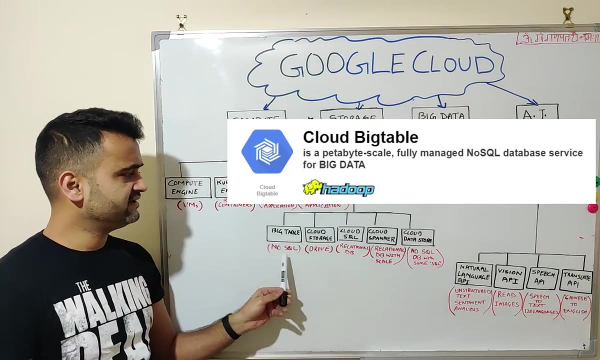 cloud storage service. we have various services, various products provided to crunch your data, to massage your data, to store your data. so let's understand how it is done. the first major product provided under storage is bigtable and, as i have highlighted, this is a no sql database. so people 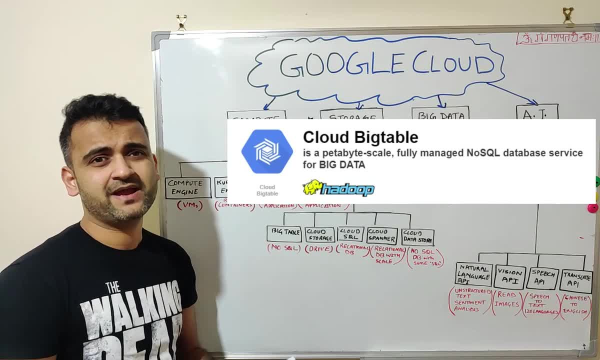 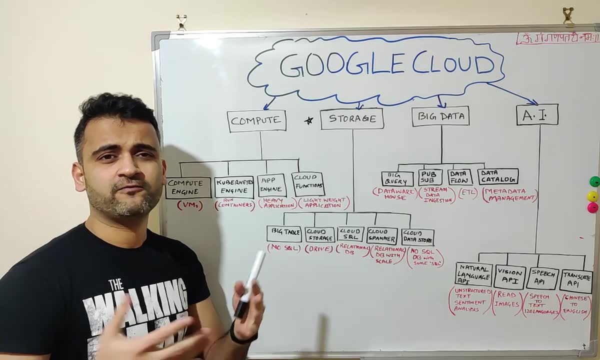 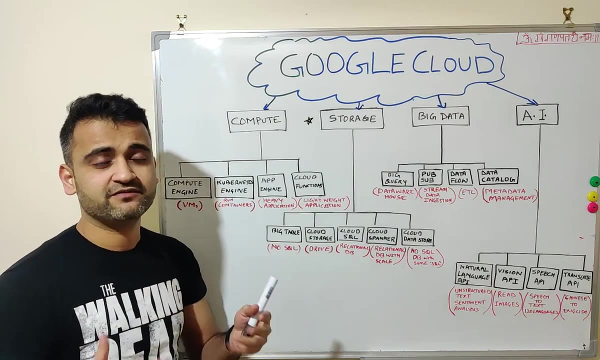 who don't know no sql database. just from a layman perspective, it is a no sql database where you cannot apply the concepts of us traditional relational databases. so data which is not structured, which is big data, which is simple, sparsely populated, which is not acid compliant, all such kind of data can be stored in a big table. 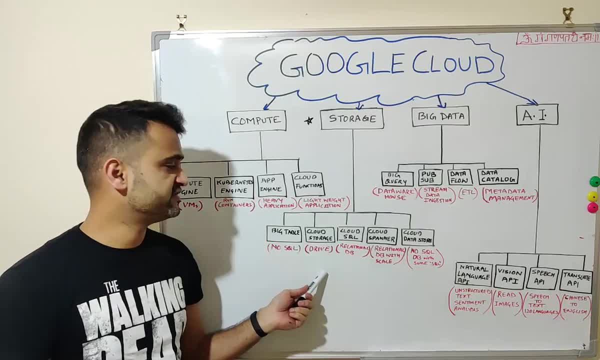 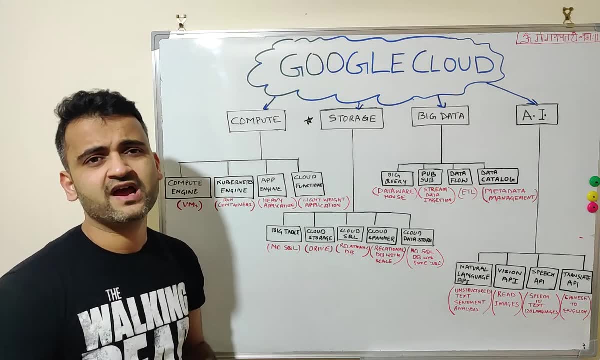 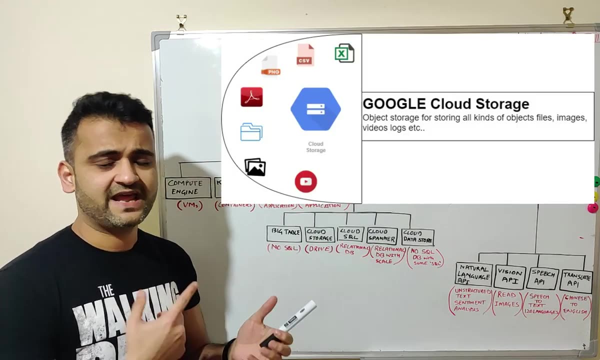 or any other big data database. moving on cloud storage, i have highlighted this as a drive because you can simply consider cloud storage as your c or d drive on your laptop. it is an object store where you can store all kind of objects like images, files, excel, csv, whatever files. 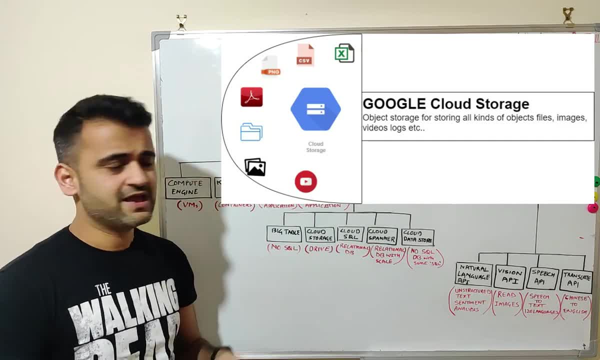 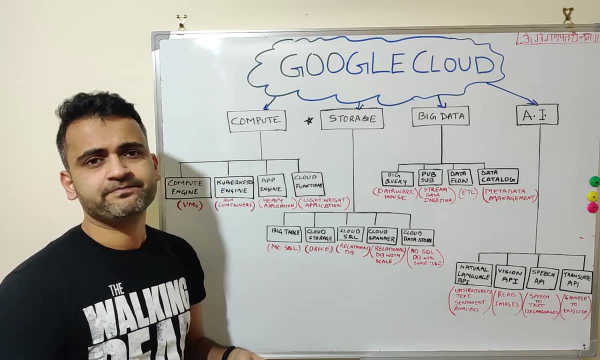 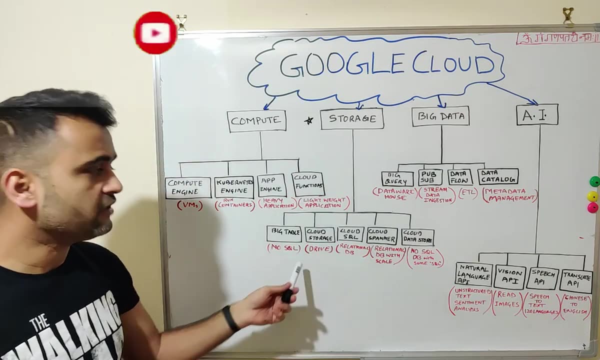 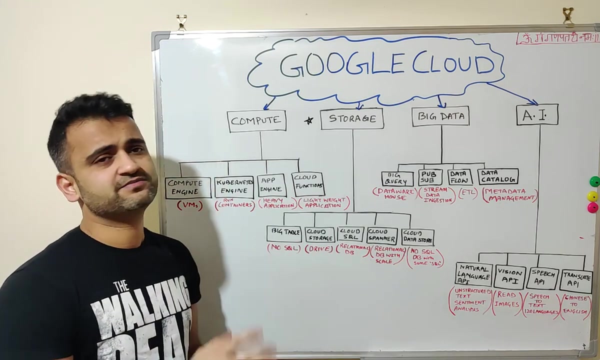 you want to store, you can store under cloud storage. it has a concept of buckets, so within storage you have multiple buckets, like you have folders within a drive, and within those folders or within those buckets, you can store your files, images, whatever. so it is pretty straightforward. it is also gives you exabyte of capacity. so, capacity wise, all these products are. 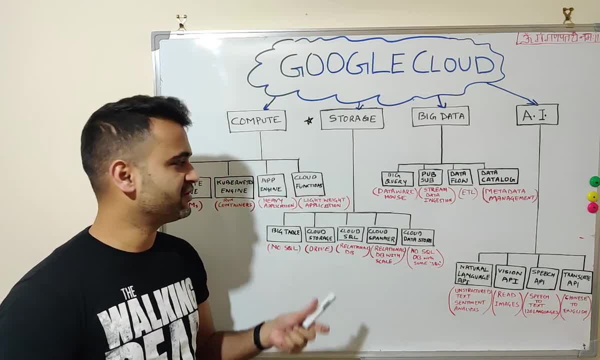 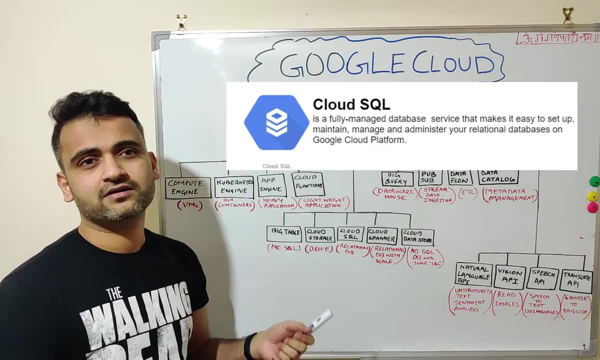 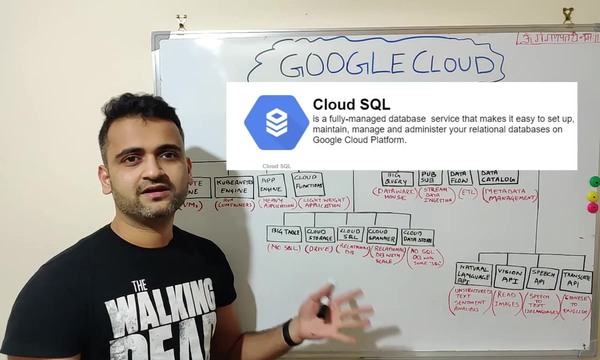 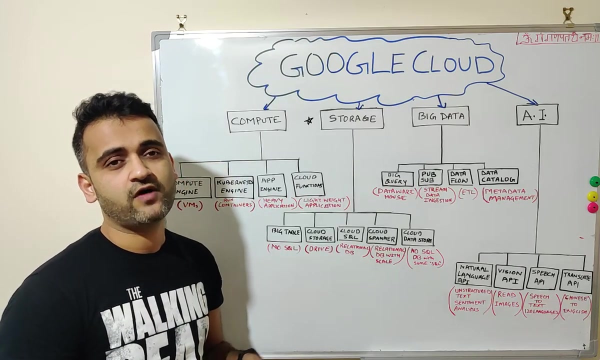 very, very good cloud sql. now this can be easily relatable because sql is a relational database uh product which can be easily correlated with our day-to-day relational database like oracle, mysql. so it is very simple: all the relational database needs can be fulfilled by cloud sql. obviously, cloud sql has some limitations in terms of how. 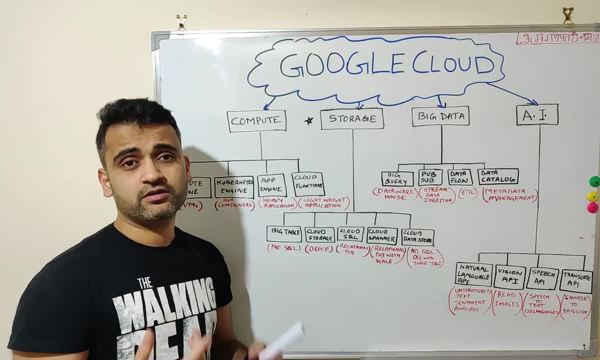 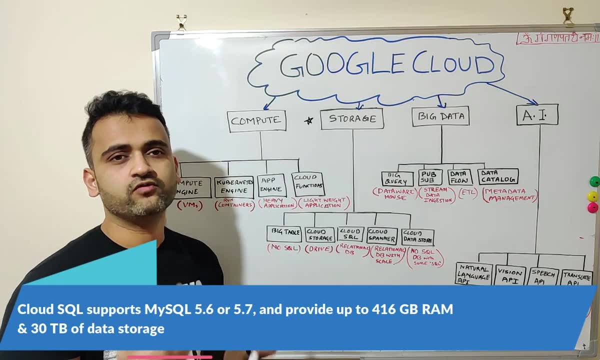 much data it can process, because it is. it is based on my sql database but, yes, it is very, very efficient if you, if your data needs are not very high. so it is very, very efficient if you, if your data needs are not very huge and if you want to run your relational database loads and if you want to do your database. 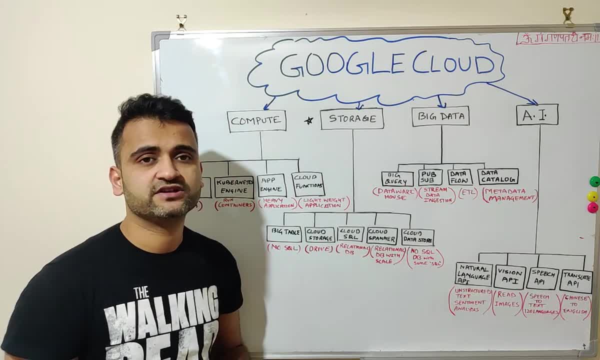 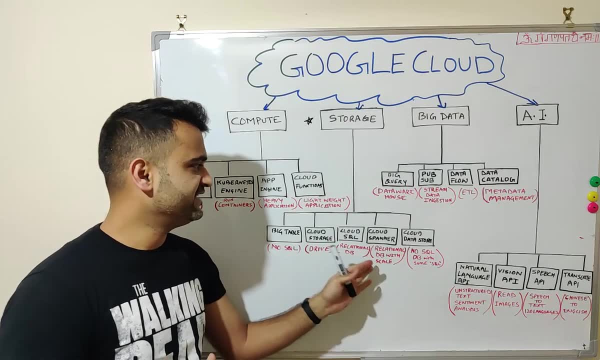 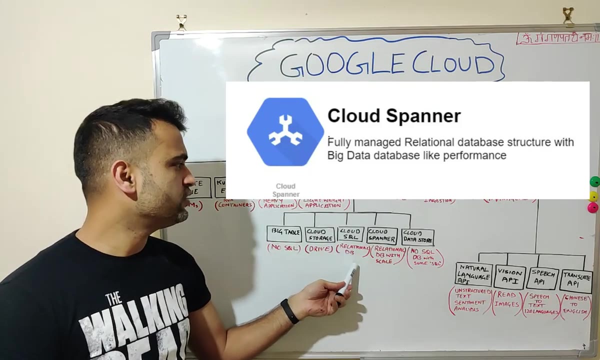 analysis, a relational database analysis, then cloud sql is a good product. cloud spanner- cloud spanner can be considered as a big brother for cloud sql. so cloud spanner is a relational database with big data capabilities. so you can consider it as if you combine cloud sql and big table. 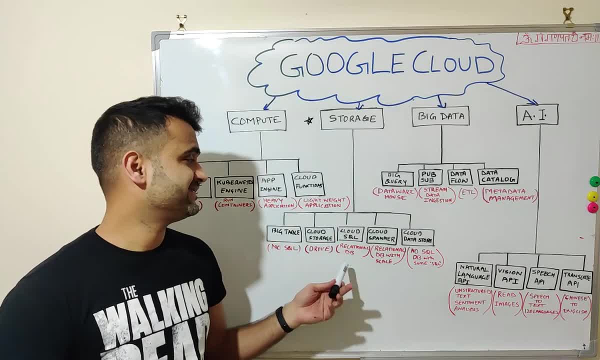 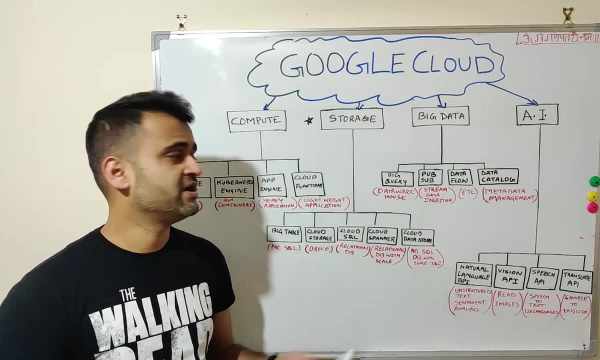 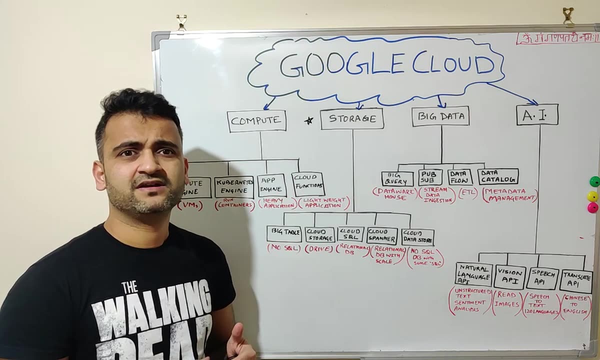 capabilities. that makes a cloud spanner. so cloud spanner is similar to cloud sql with massive scale and massive capabilities to run big data loads with sql support. so cloud spanner should be your go-to product if you have massive database needs with massive amount of data and 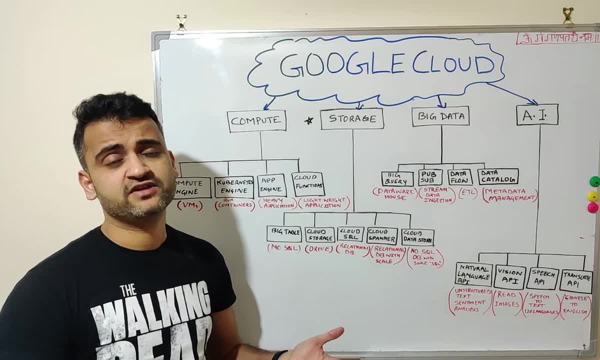 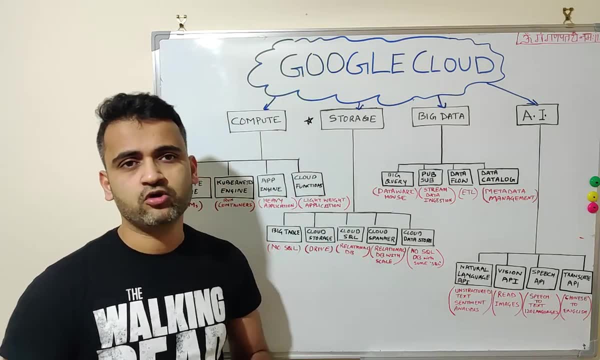 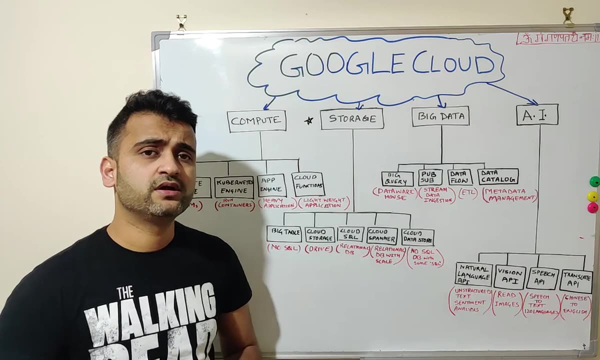 massive performance. but you have a relational database and you have a relational data which needs to be uploaded or used in google cloud platform, then cloud spanner is a product for you. but for every normal database needs you can go with cloud sql. cloud data store is again you can say is a subset of big table. 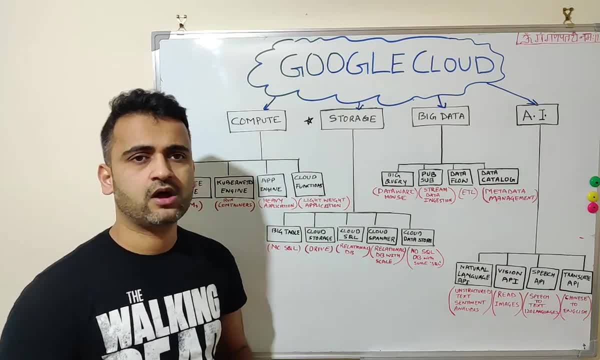 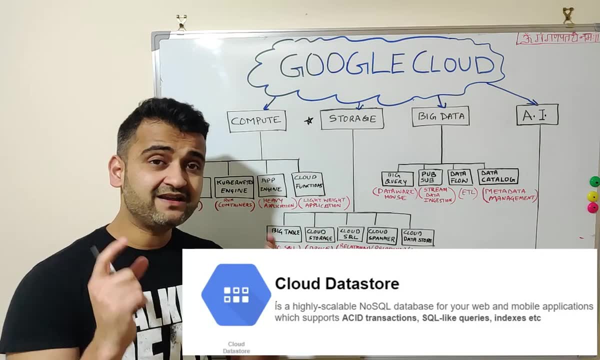 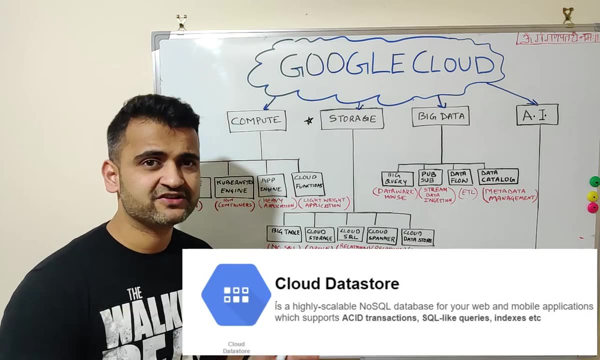 because what big table cannot provide is somewhat provided by cloud data source. so cloud data store sits on top of big table technology, but with slight sql support. although it is a no sql database, it still gives you some flexibility of using sql and do your analysis using sql queries. 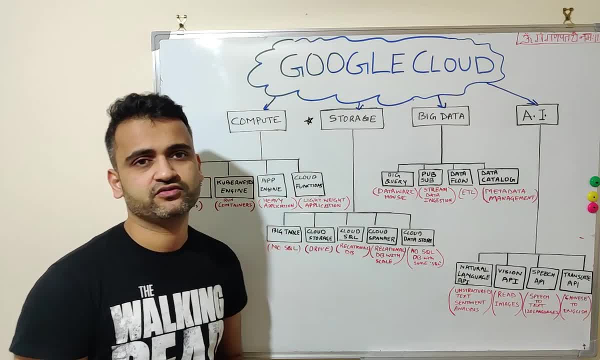 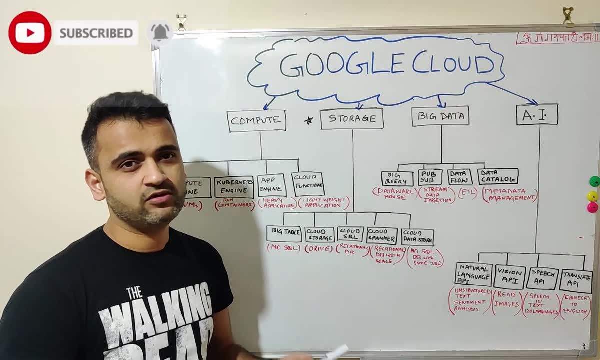 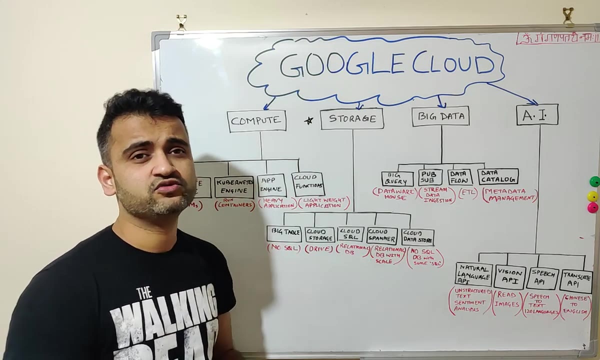 is the major difference between- uh, big table and cloud data store. again, friends, we are not going into very deep details of these products because it would be really impossible in one video. so in future videos we'll target every product and every service one by one and we'll take various use cases. 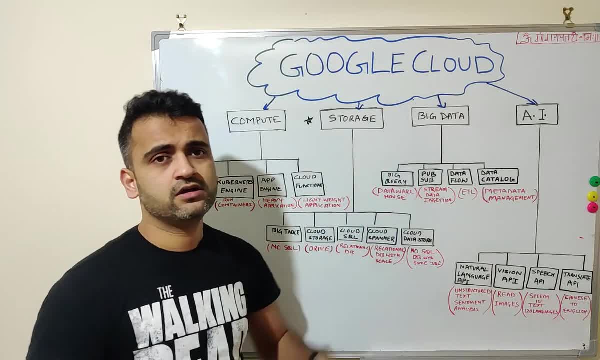 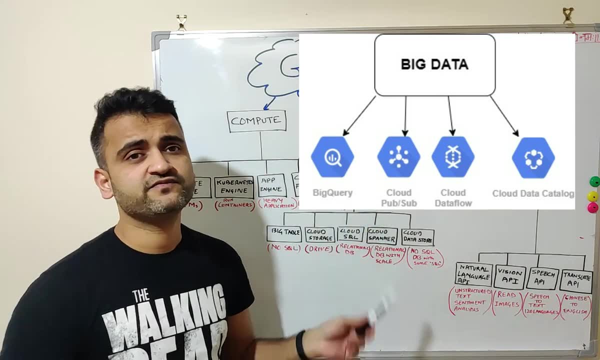 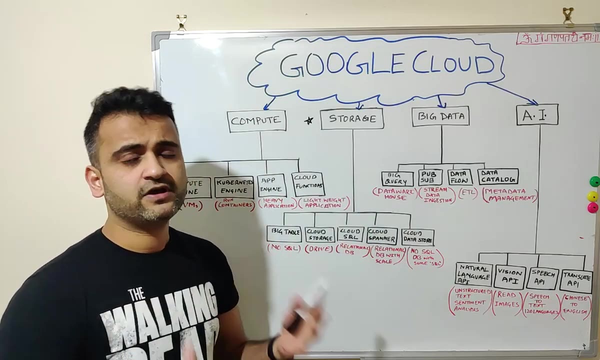 and we'll understand it one by one. moving on, the next category, which is again a very famous category, is big data. so big data in under big data. the most famous product, which is the usp of google cloud, is bigquery, because bigquery is google cloud platforms: data warehouse. 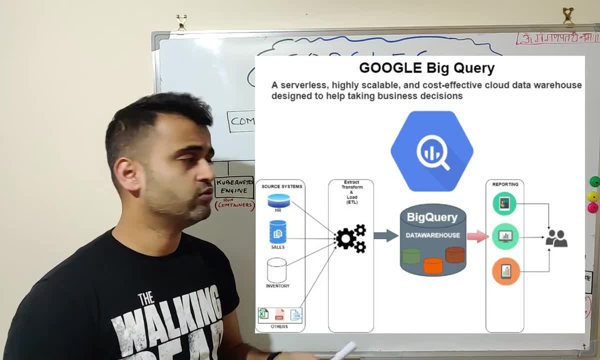 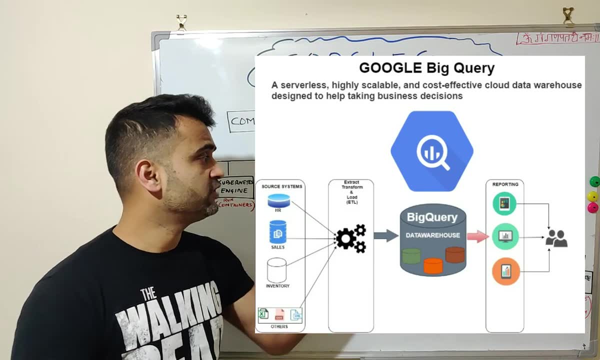 solution where you can run your data analytics and data loads and you can store your massive amount of data under data warehouse. so whatever data warehouse or data lake needs you have, you can get it fulfilled by using bigquery. if you don't know about data lake, please go and check out. 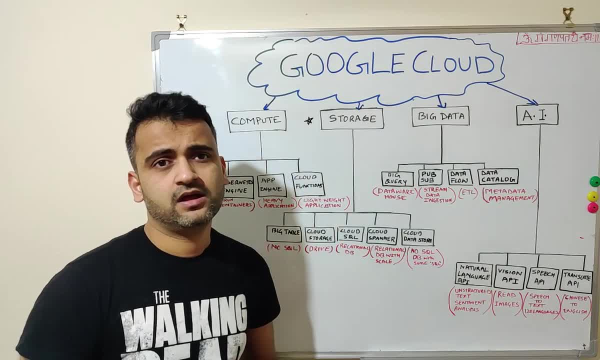 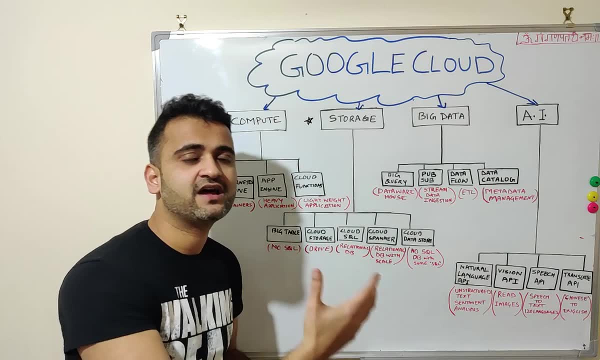 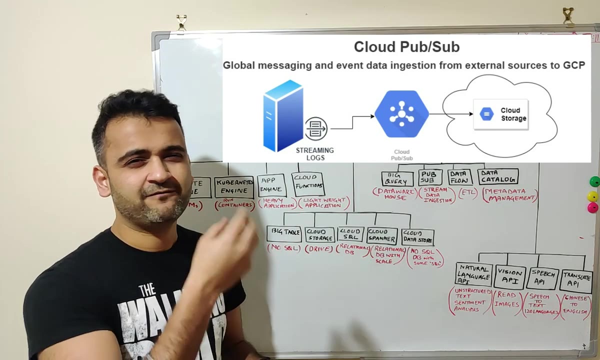 my video which i have made on the same topic, pub sub. this is an interesting name, and this particular technology is used to ingest streaming data into the google cloud platform. imagine a server which is running and generating logs every few milliseconds and those logs needs to be captured. 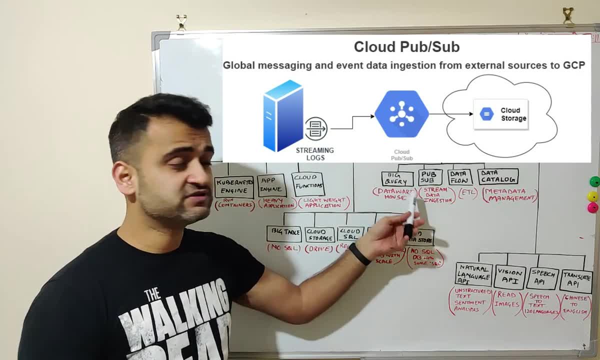 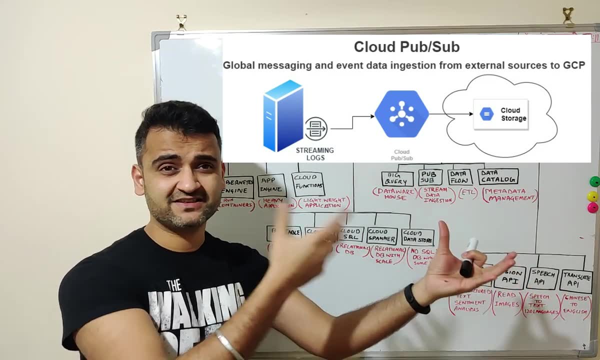 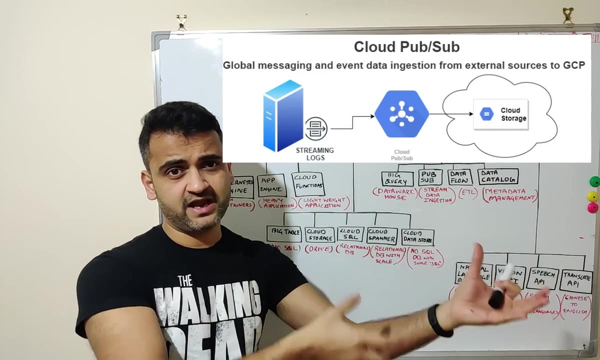 and analyzed. so in that, in that case, pub sub is a very good middleware which can sit between that particular source, which is generating huge amount of data every second- so that is a streaming data, live data- and pub sub can make sure that that data can be fetched from that source and ingested into google cloud platform. so it is kind of a middleware. 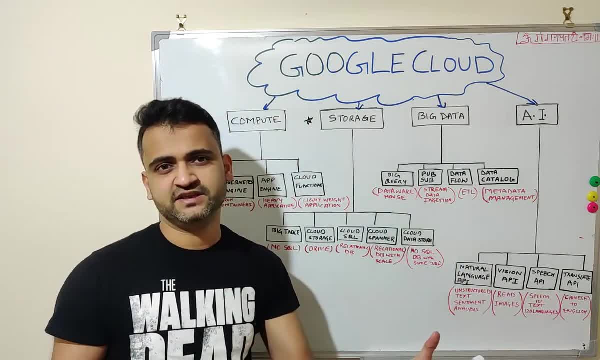 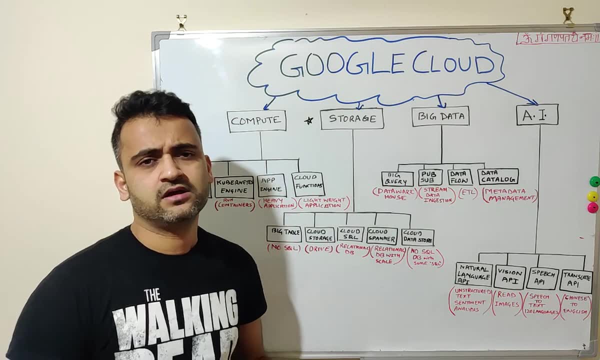 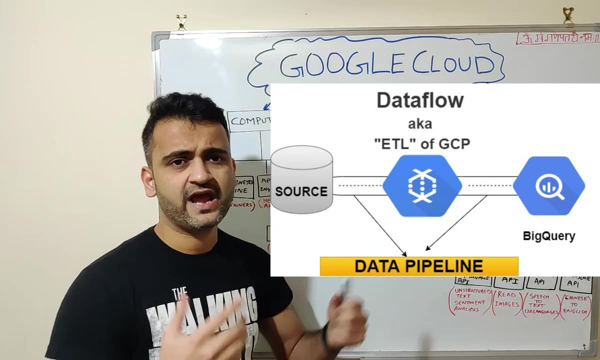 which sits between source and gcp, which is google cloud platform, data flow. data flow can simply be considered as an etl product, like any other etl product: uh, informatica, data stage, sap, data services. this also helps you extract, transform and load data. it helps you extract batch. 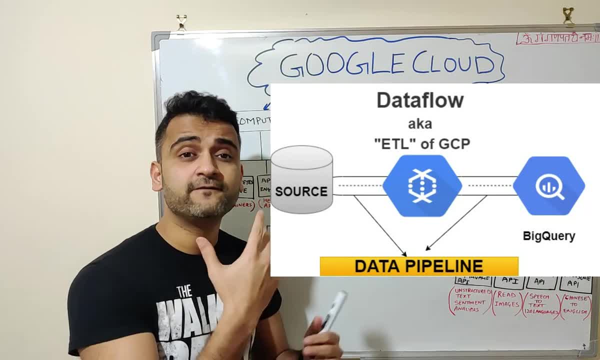 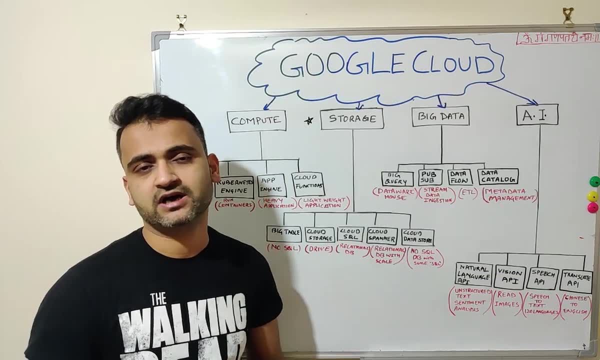 data and the streaming data at the same time, and you can create data flows within gcp and you can process your data and massage your data and then load it into the target. so this is pretty much what an etl tool does. so if you want to, 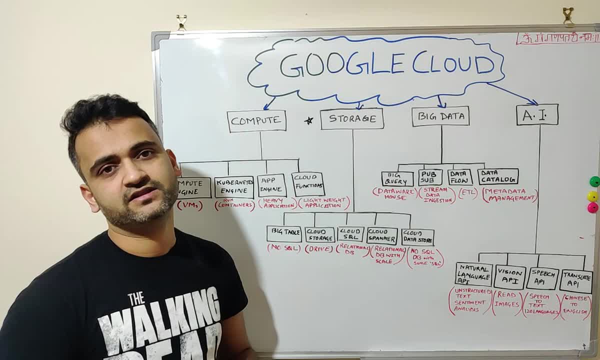 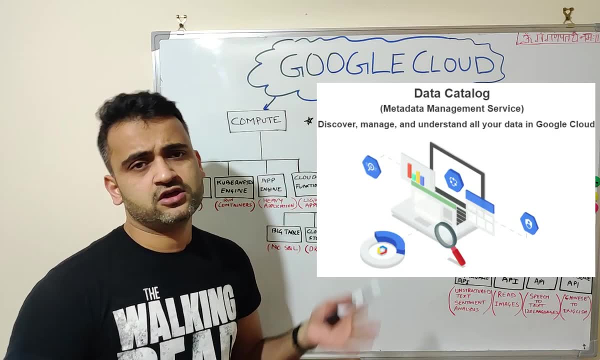 any time understand data flows. you can simply correlate with an etl product data catalog. data catalog, again, is a metadata management service. so, as you know, you need to know your meta data in order to understand the flow data information and you can summarize the flow data in your data panel. 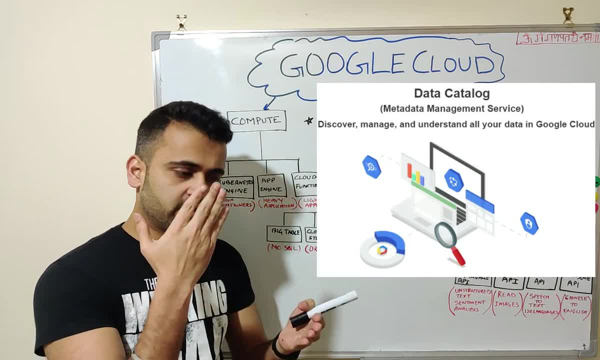 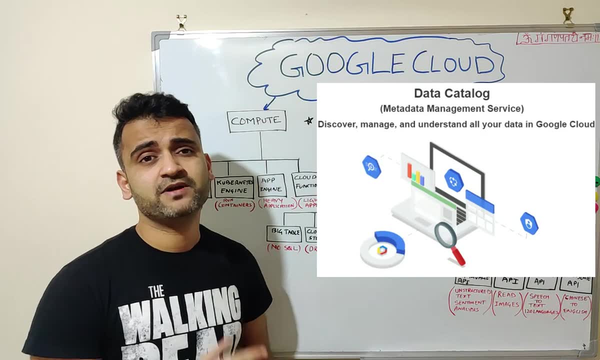 understand what is floating around your cloud platform. so if you want to understand what is there in your data warehouse or in your data lake, then your metadata management has to be top-notch. else, as i have explained in my data lake video, your data lake can very quickly become a data. 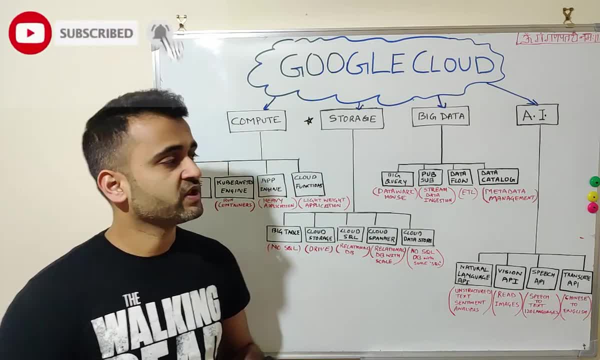 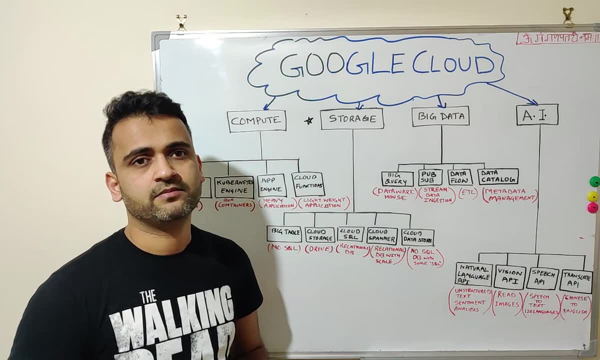 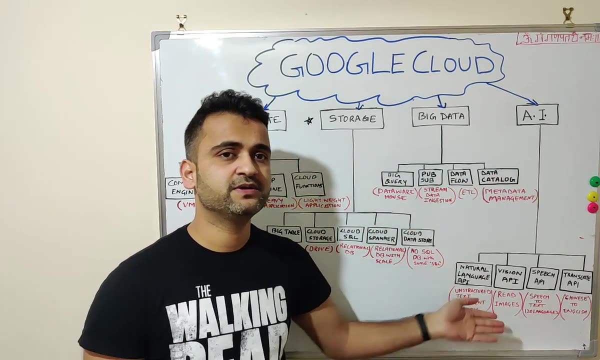 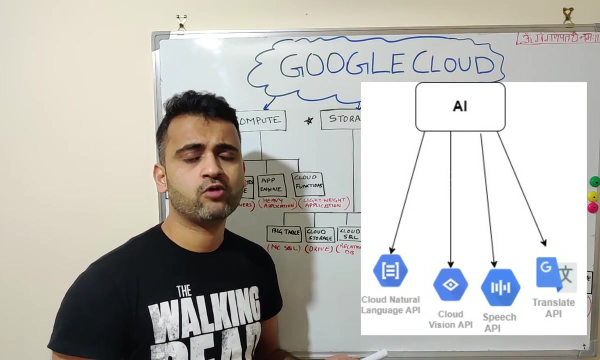 swamp if you do not have a proper metadata management. so that's why data catalog is a very, very efficient technology and product to make sure that you manage your metadata properly. so, moving on to the last category, which is artificial intelligence, under this we have multiple products provided, so all these products are basically based on different auto ml models. 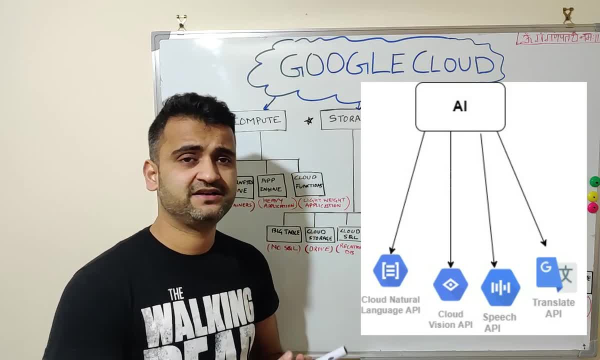 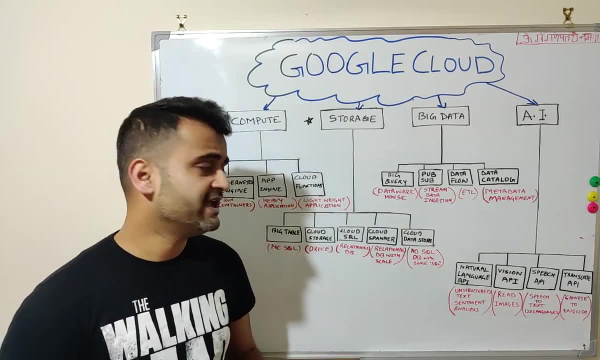 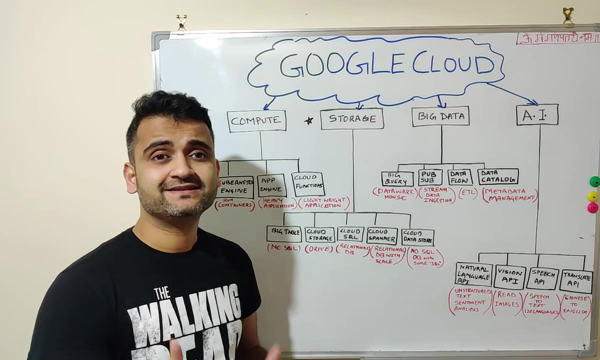 which is automatic machine learning models which are developed by gcp and are readily available for the business to utilize. so the first one in this category is natural language, api, and this is a very famous product to do sentiment analysis. sentiment analysis can be quickly understood by an example of doing twitter analysis during. 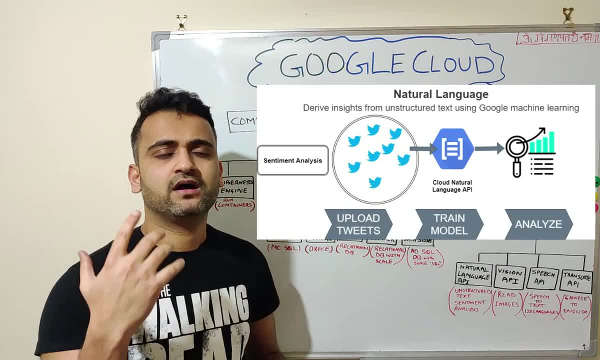 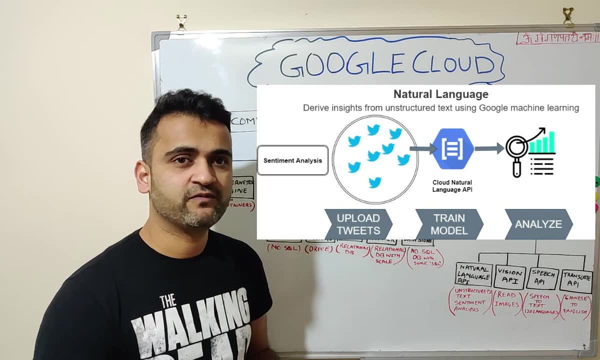 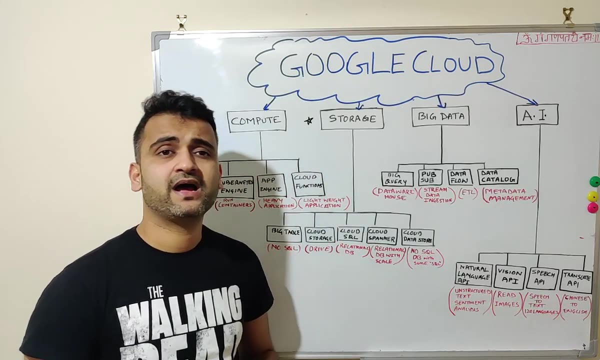 an election poll. by reading the twitter messages and tweets, you can understand which particular party is leading, which party has a better chance of winning. so all these kind of analysis can be done using a machine learning model which is provided by a natural language, api, and by the. 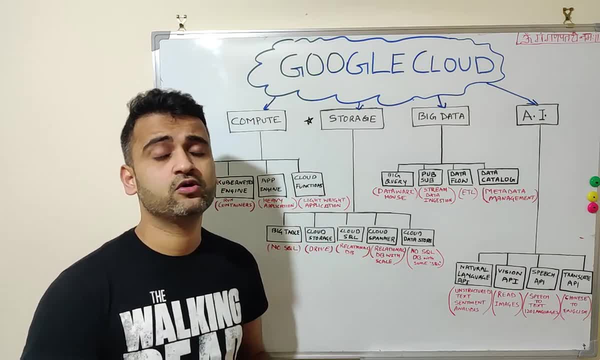 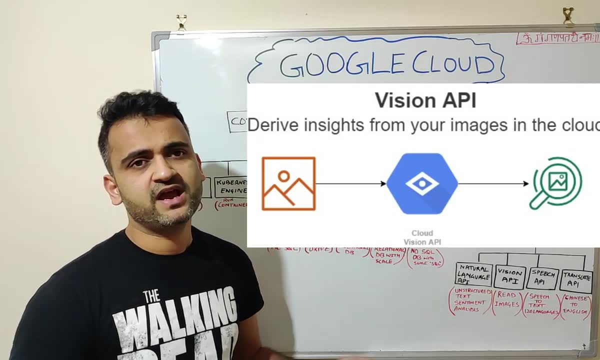 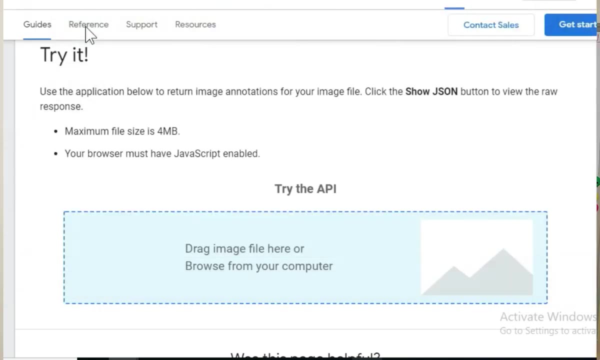 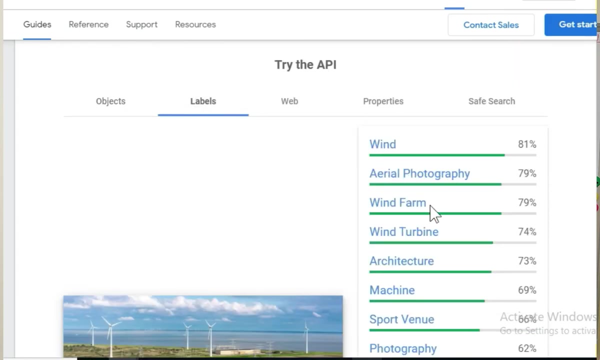 way, if you don't know api, i i again have made a separate video on api, so go check that out. vision api, as the name suggests, this particular api and machine learning model helps you read images. so if if i upload an image under vision api, by just reading that image the gcp platform can help you identify the data points which are. 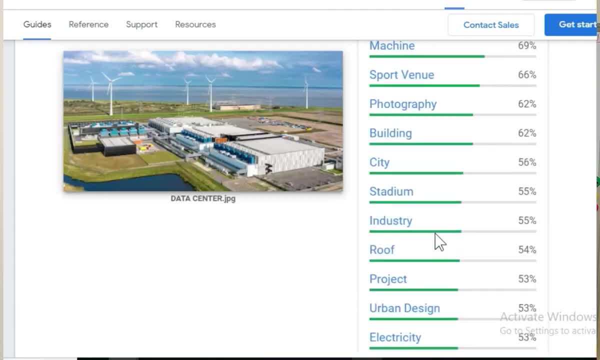 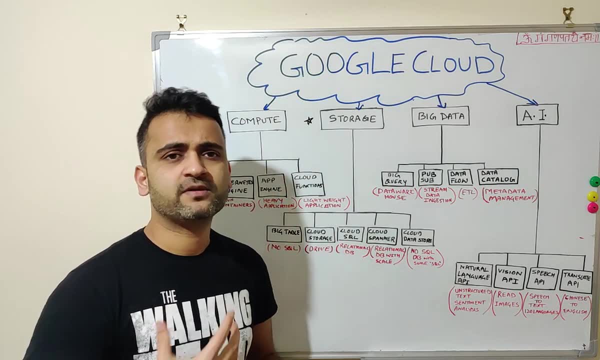 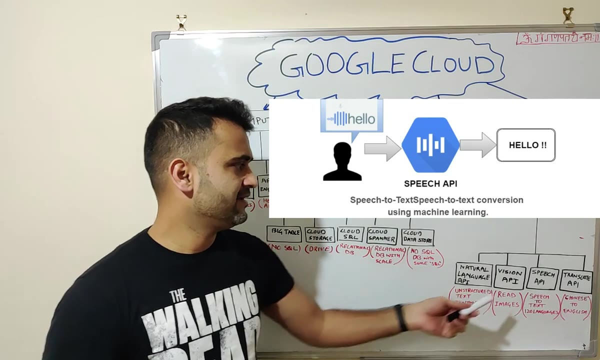 related to that particular image, so it is very, very efficient for image data processing. speech api helps in converting your speech. so suppose someone is speaking and at the same time you want that particular speech to be converted into a text, then that in that case this particular api and machine 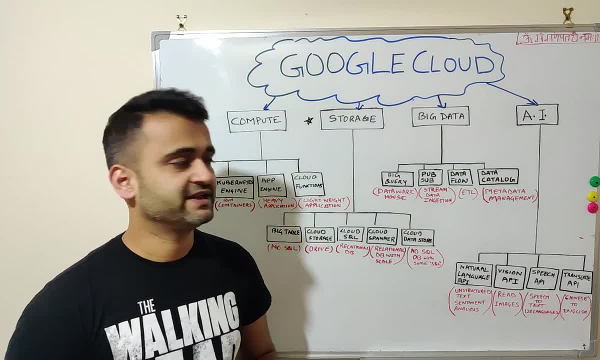 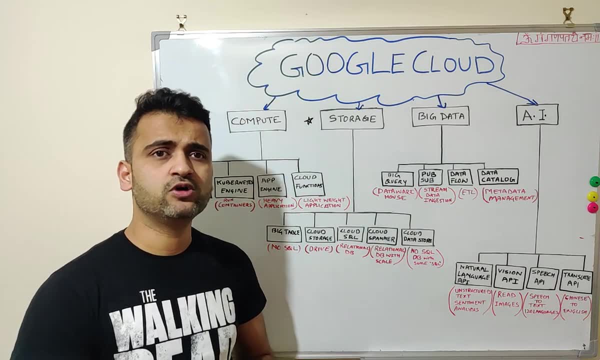 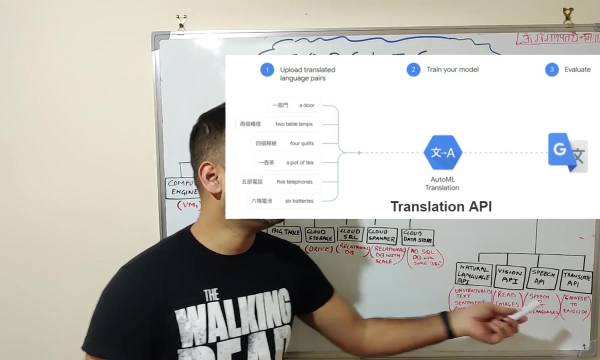 learning model comes handy and it helps you do that analysis: translate api. so this again is self-explanatory. translate api helps you convert one particular language into another. so suppose you have something written in chinese, you can convert it to another language and then you can, you can feed that into this translate api and it can come convert it into english or any other. 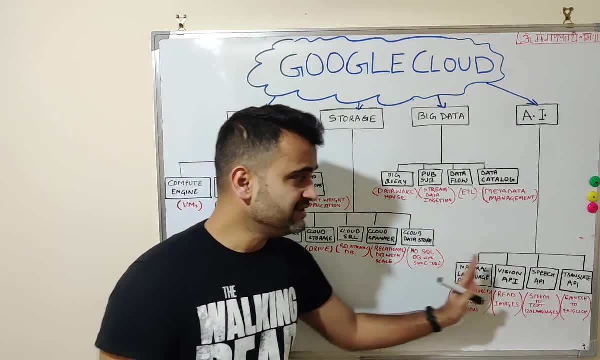 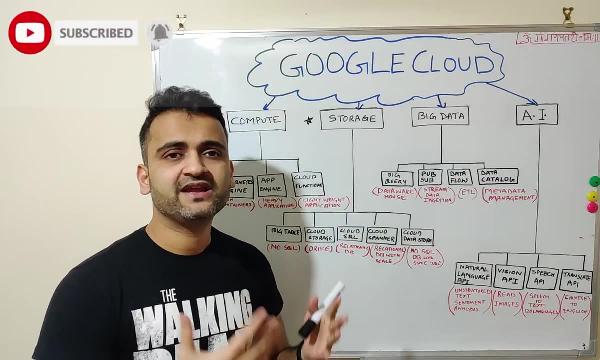 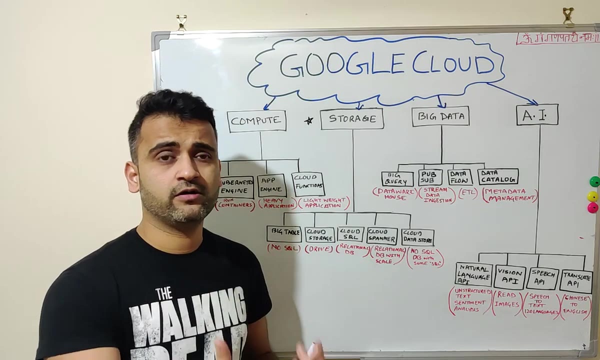 language of your choice. so all these apis and all these machine learning models needs data to train uh itself. any machine learning model cannot work unless it has a training data and based on that only it can run those statistics and come out uh with some predictive analysis. one very good uh product which has been added recently is video translation.